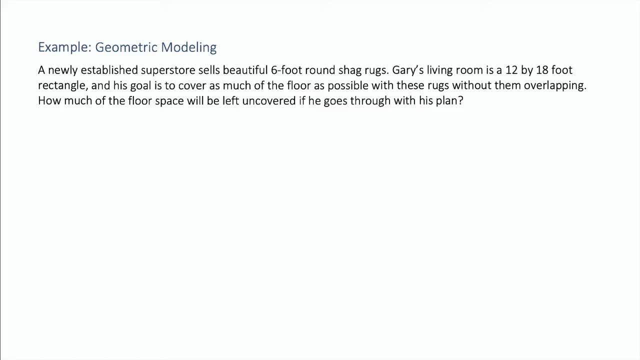 will be left uncovered if he goes through with his plan. Let's draw a picture here. We've got a rectangle, okay, a 12 by 18.. So 12 by 18.. And of course, it doesn't have to be a perfect. 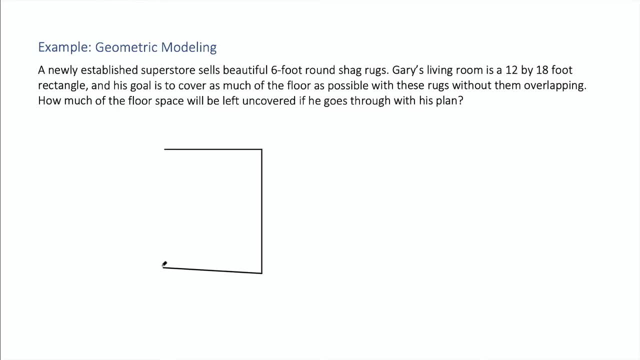 rectangle that we draw. There we go 12 by 18.. So there's Gary's living room And he wants to cover this with some rugs. Now we've got six foot round rugs. Now when we say we have a six foot rug, that's going to be the diameter. okay, It's. 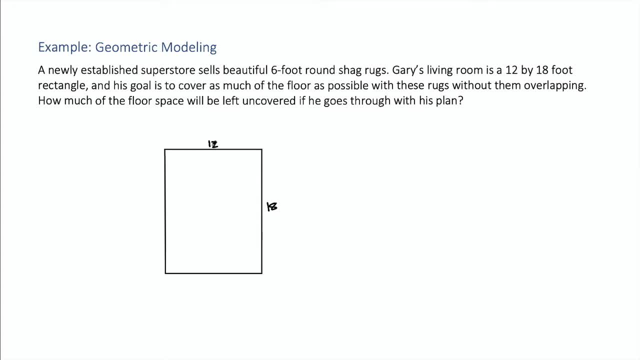 going to be six feet across, So we can go ahead and draw that. Now, since we've got 12 feet across, we're going to be able to fit two circles side by side here. Okay, there's one, It's probably. 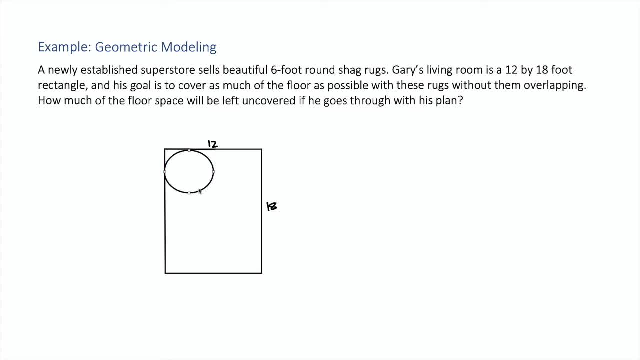 going to be a little bit bigger than that. There we go, And then another one, Okay, another just just as big, same size, Okay, so we've got there's two side by side rugs, And so that goes all the way across And it's 18 feet down, which means we're going to be able to. 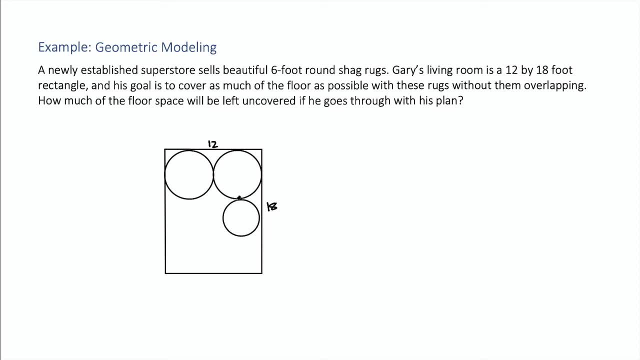 fit three. Okay, there's, oh, there's one, And of course I am not the greatest artist. There's one And there's another one, So obviously I didn't make my rectangle big enough. I'm going to be. 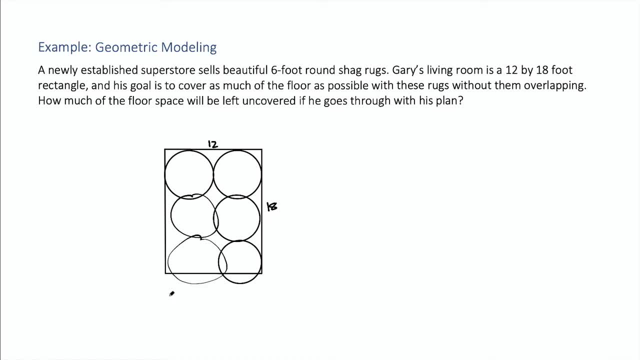 kind of sloppy here. So I've got, I've got six rugs here. Now if I wanted to be very, very precise here, I could go ahead and and delete, delete. I can erase these, These and then just copy And. 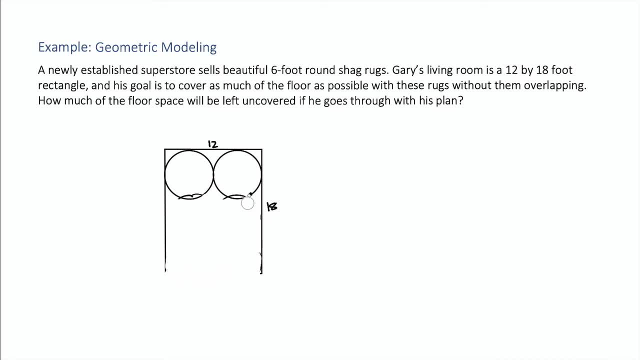 I'm going to go and do that just so that we're very, very clear about what, what is happening here. So these two, these two things here, those two circles, we're gonna go and copy those And we're gonna go and paste them And then put them down. 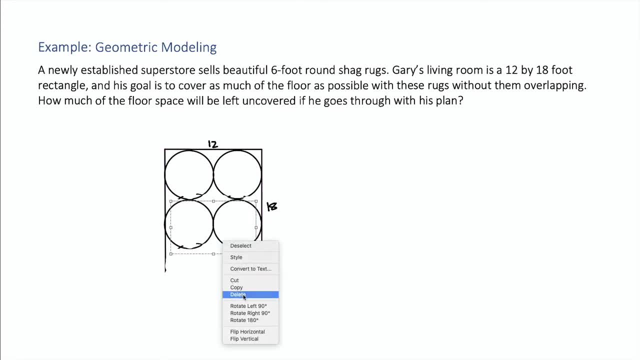 And then, same thing, we're going to go ahead and we can copy those and paste them and write underneath: Okay, so that that's now the proper ratios. Okay, All right, so there's our. there's our room, with the six rugs that we're able to fit here. Now we want to know how much floor space. 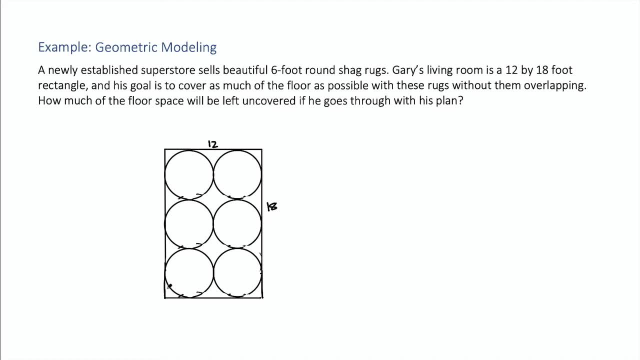 is left uncovered. So it's easy to get the area of the rectangle Okay. the area of the rectangle is well length times times width. that's 18 x 12. And that is 216.. It's also easy to get the area of these circles area of the 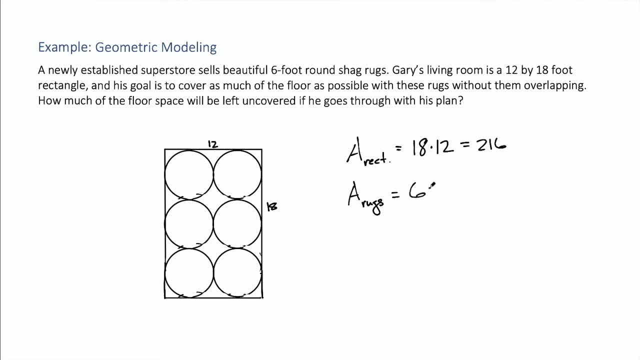 rugs. Okay, Well, there's six rugs times the area of a circle is pi r squared, pi times r. and this case it's a- remember, it's a six foot rug, so R the radius is three feet. that's three squared. okay, so this is nine times six, which is 54. all right, that is 54 pi. 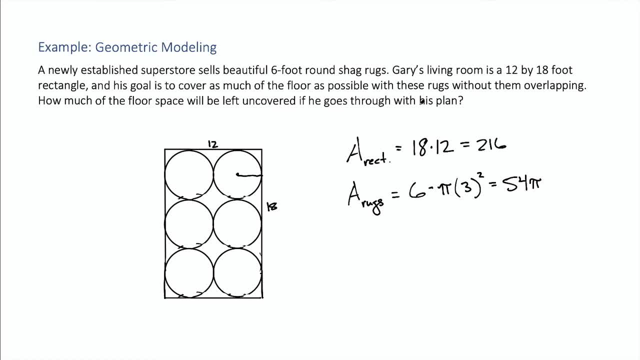 and so the I'm looking for the area of what's left uncovered, okay, so what we're actually looking for here is this little area and this little area and this little area. okay, all the way down, that's what we're looking for. so, in order to get that, all we need to do is take the total area of the floor and 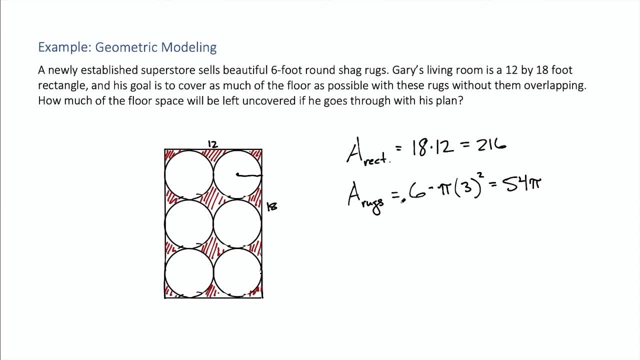 subtract the area of the rugs and we have those two areas so uncovered. the area that is uncovered is 216 minus 54 pi and uh, we can go. we can leave it like that, or, if we want a decimal, we can go ahead and and and type this into a calculator, or we could use an approximate form for pi. 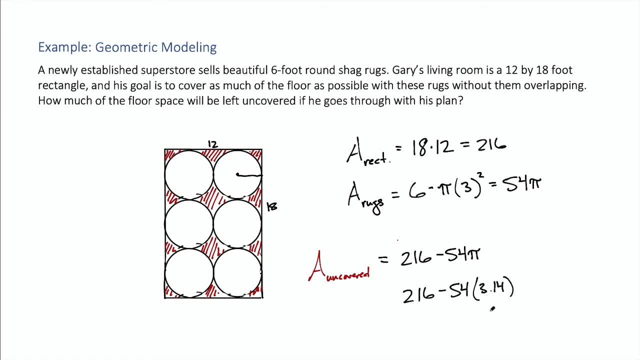 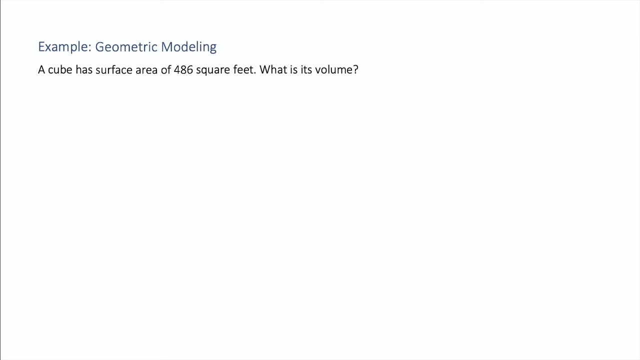 pi is about three point one, four, and this is going to be in square feet, because all of our units are in two feet. so that's the square feet. a cube has a surface area of 486 square feet. what is its volume? let's draw a quick.